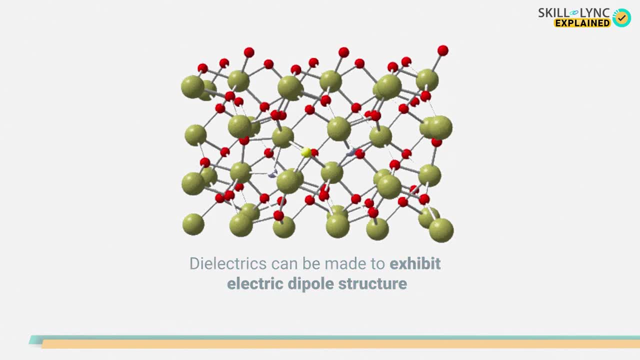 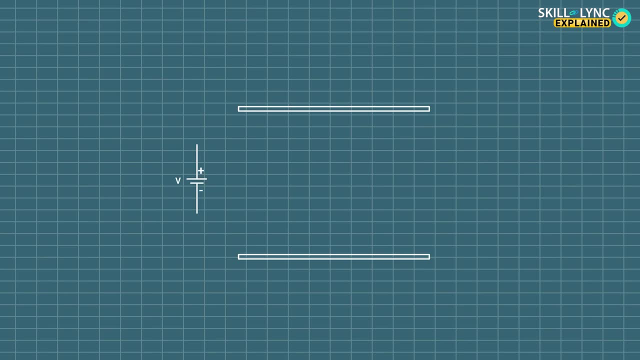 But it can be made to exhibit electric dipole structure. Let's see how this happens. Assume we have two conducting plates separated by a particular distance. When it is connected across a voltage, the plate connected with the positive terminal will get accumulated with positive charges. 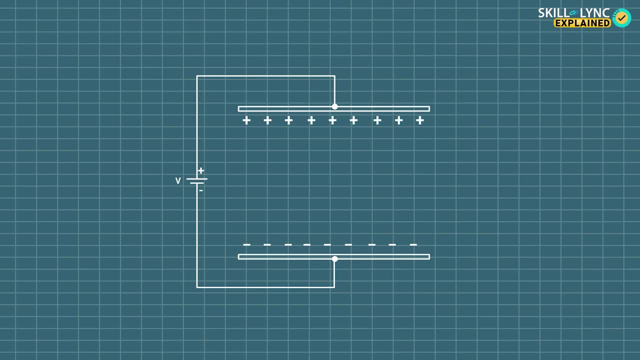 And negative charges will accumulate at the other plate. This remains since there is no medium in between to conduct current. Now let us place a dielectric material in between the plates. At this time, positive charges in the dielectric will accumulate near the conducting plate. 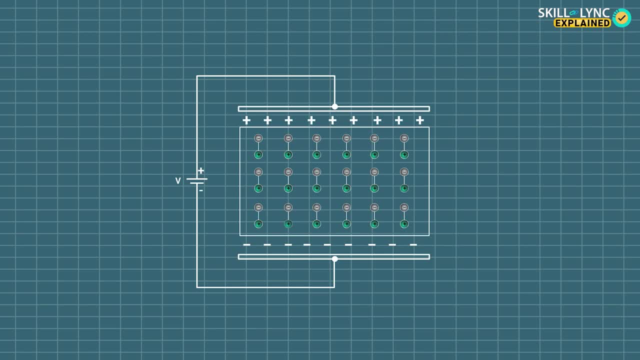 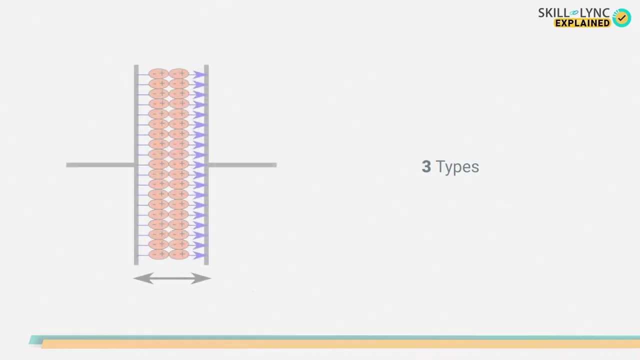 with negative charge, whereas the negative charges in the dielectric accumulate near the plate with positive charge. The process by which the dipoles in the dielectric will accumulate will be called a positive charge. electric align themselves when an electric field is applied is known as polarization. 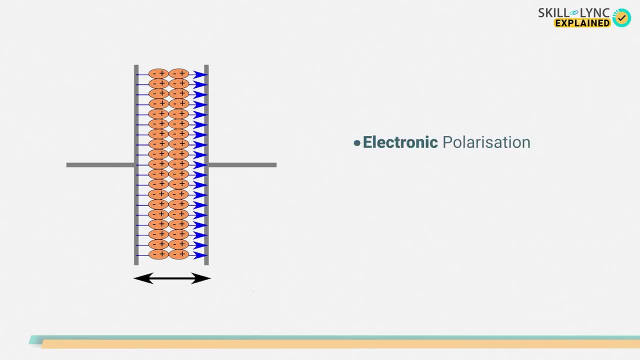 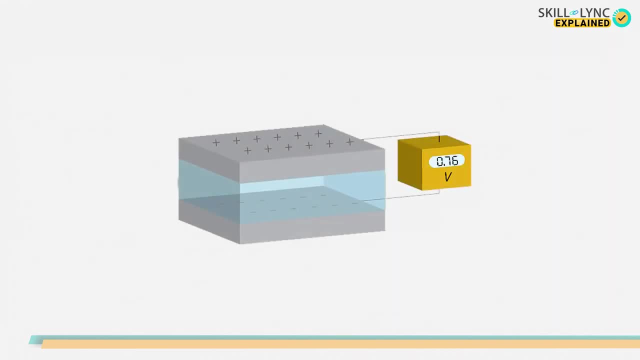 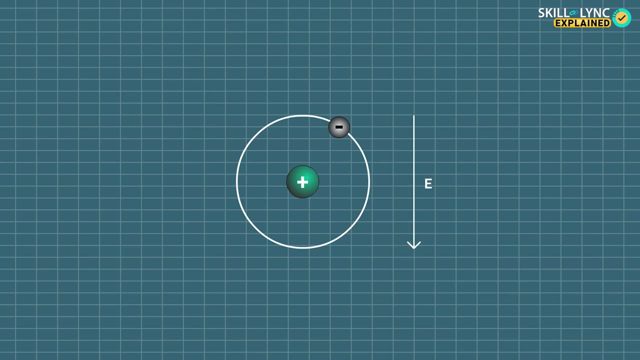 Polarization is of three types. They are electronic polarization, ionic polarization and orientation polarization. A dielectric material exhibits at least any one of these three types. Electronic polarization is the type in which the center of the negatively charged electrons displaces from the center of the positively charged nucleus. This polarization is noted. 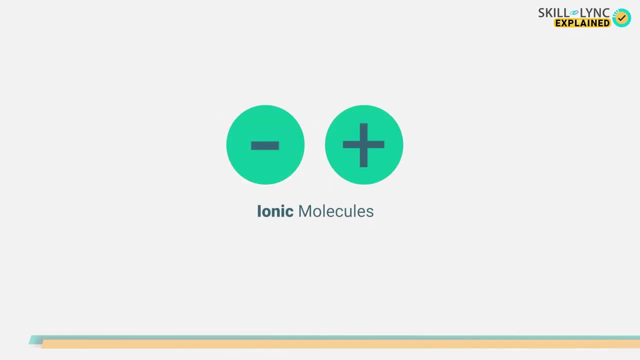 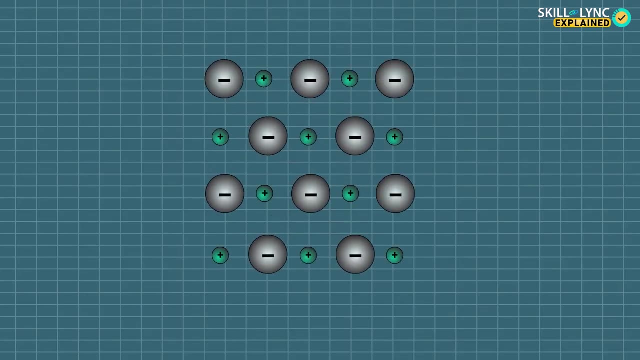 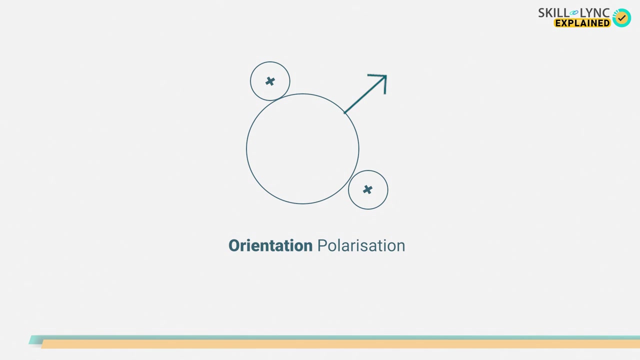 in all types of dielectrics. Ionic polarization is found in ionic molecules. When a field is applied, the cations move in one direction, whereas the anions move in another direction. The third type of polarization is the orientation polarization. This type is only found in dielectrics. 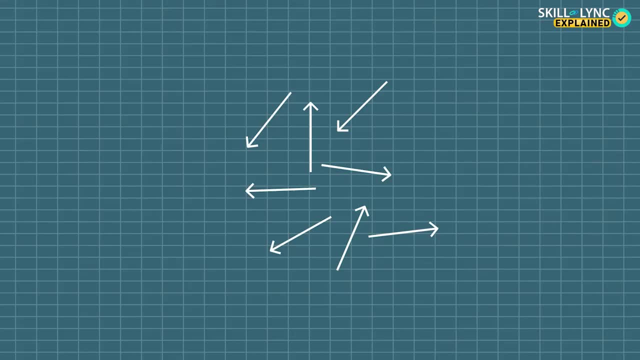 with permanent dipoles Here. the electric dipoles in the dielectric will rotate in the direction of the applied field. Thus the total polarization in a dielectric will be the sum of all three, ie electronic, ionic and orientation polarization. 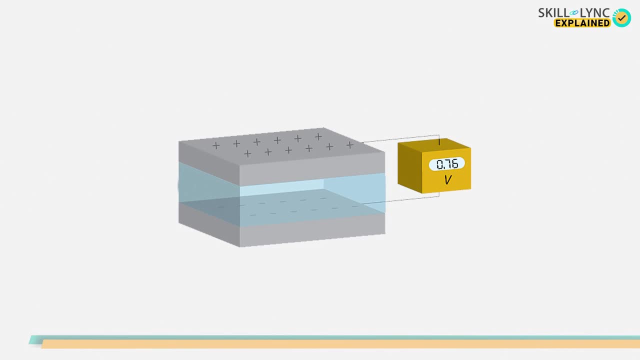 For selecting a dielectric material, its properties should be carefully considered. The first one is the permittivity of the dielectric material. Permittivity is defined as the ability of the material to store electric values. The following material is artificially applied to a dielectric field and the output is also: